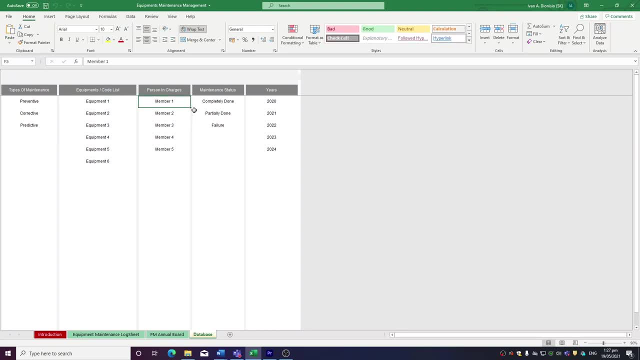 input the people in charge, like the technicians or mechanics, that you have the maintenance statuses and years in the periods that you want. It's important that you don't have to Don't miss anything or anyone here, because the data here will be used for the drop-down. 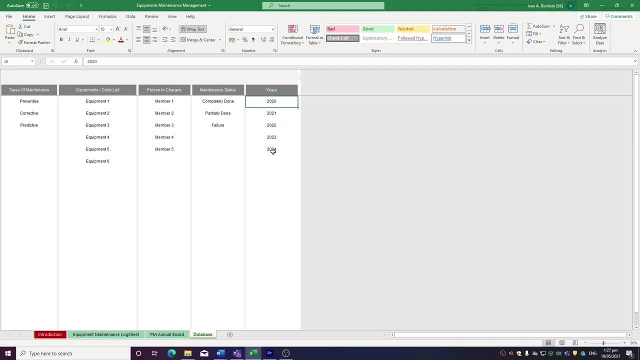 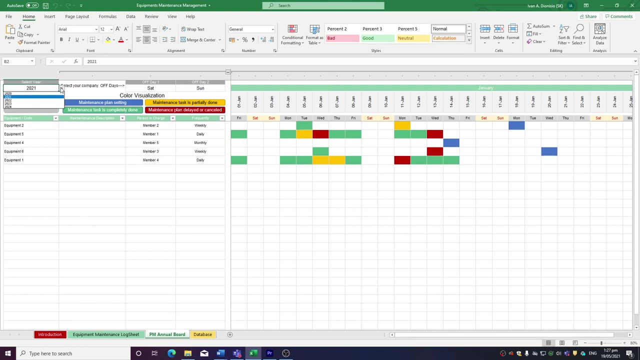 lists in the following tabs. Moving to the PM Annual Board tab, we can select the year using the drop-down. Then you input your two off days of the week. Usually we'd have Saturday and Sunday off, but in case your business differs, say it's. 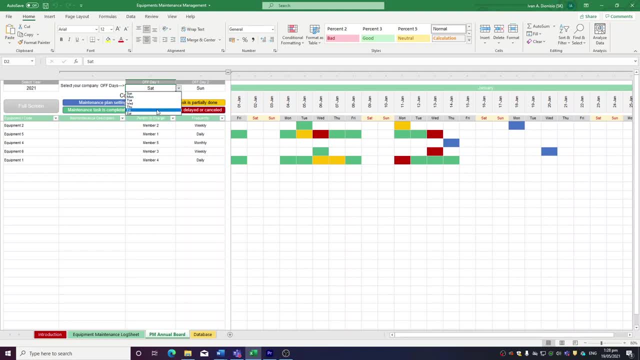 Friday and Saturday. you can change it using the drop-down and the off days would automatically reflect on your day rows in the calendar. After that, we input the pieces of equipment we want to keep track of using the drop-down: A description of the maintenance task, the person in charge of the task and how often. 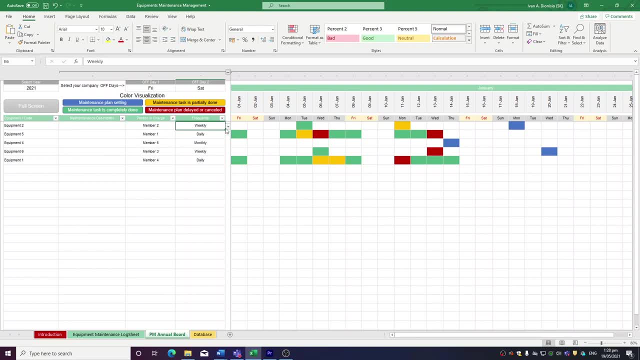 the maintenance job is performed Up here. we have a legend on color visualization. So there's basically four categories you can set as your status for the different jobs. To the right, We have a calendar. The columns are the different dates of the week. 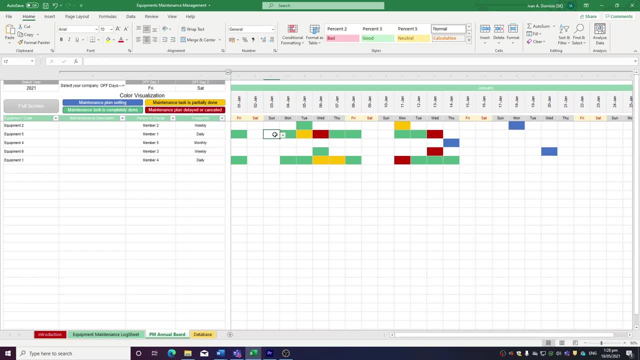 Per equipment per day. you can select the status of the maintenance job so you can keep track of the progress using the drop-down. Once you pick a status, the color changes, which reflects the colors shown on the legend. so you have a quick visual guide on the status. 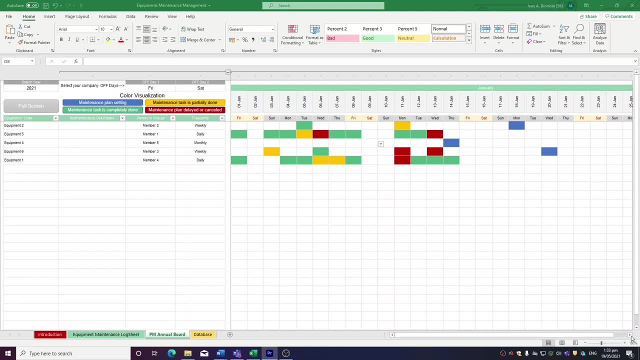 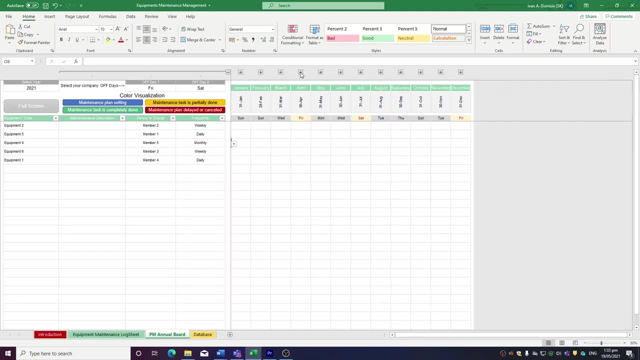 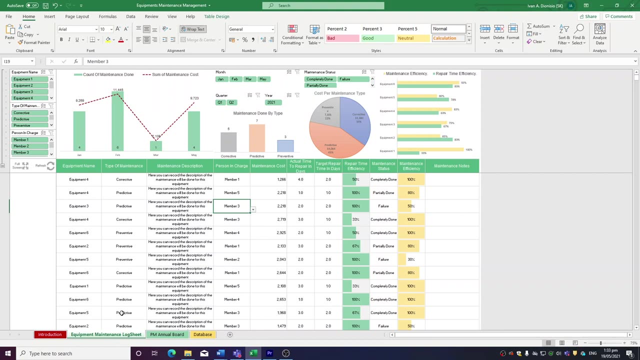 In order to see the different months in the year, you can press on the collapse and expand buttons on the top of each month. Lastly, moving to the equipment maintenance sheet, it's here where you can record your maintenance data. You log in the equipment name the type of maintenance you performed on the equipment. 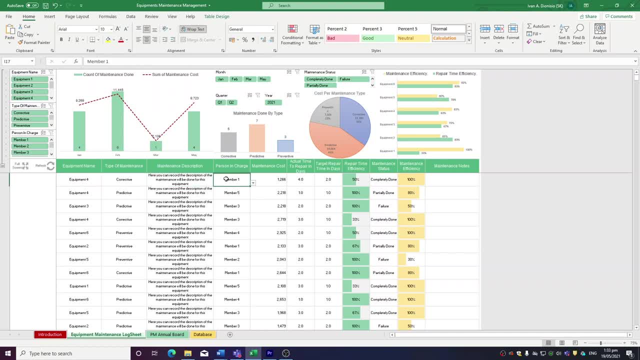 a description of the maintenance that you performed, the person in charge, how much the maintenance costs, the actual repair time in days, the target repair time in days, maintenance status and maintenance efficiency. Repair time efficiency. Repair time efficiency is computed automatically, so be sure to avoid inputting any data in. 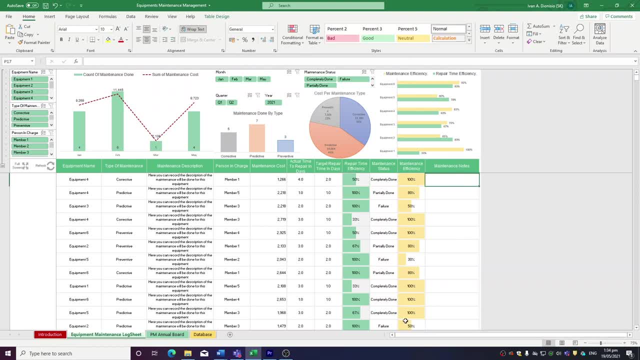 this column. There's also a provided column for any notes you might have. on the logs Up above. we have some charts to give you a visual representation of your maintenance performance. We have a graph showing the number of maintenance jobs completed per month versus the sum of 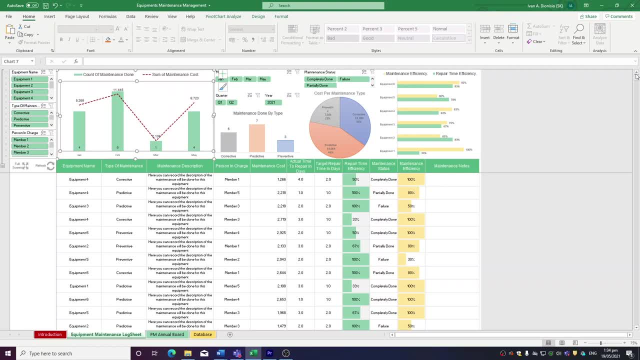 maintenance cost. This is information that you could use to make a cost analysis, to try and find out which months are more expensive to maintain equipment and even try to get the reasons why. We have a chart showing the maintenance done by type and cost per maintenance type as well. 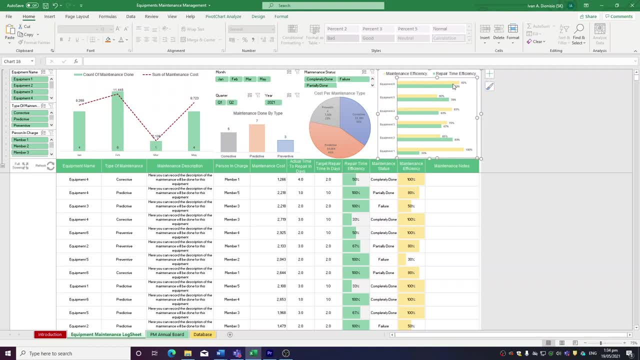 as a chart contrasting maintenance efficiency and repair time efficiency, All of which are really useful tools that you could use to gain insights to make data-driven management decisions for your business. We have some slicers here on the left, Which allows you to filter the chart data by equipment name, the type of maintenance. 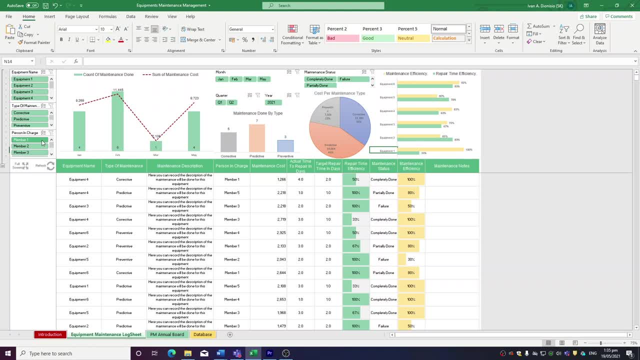 done and the person in charge. You can also filter by month, by quarter and by maintenance status. To use the slicers, just click on the criteria you want to show. If you want to select multiple criteria, simply hold down the control key. then select all. 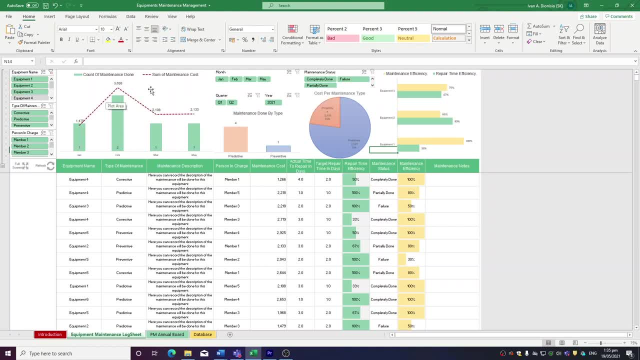 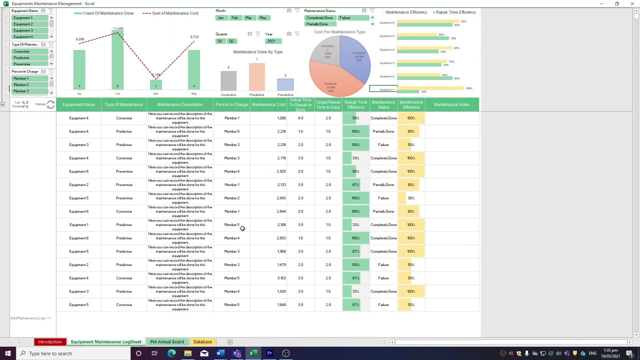 you want included. To remove the filters, You can click on the clear filter button, Then on the top right of each slicer group. Lastly, we have a full screen macro button which hides your ribbon, making your worksheet bigger and easier to read. 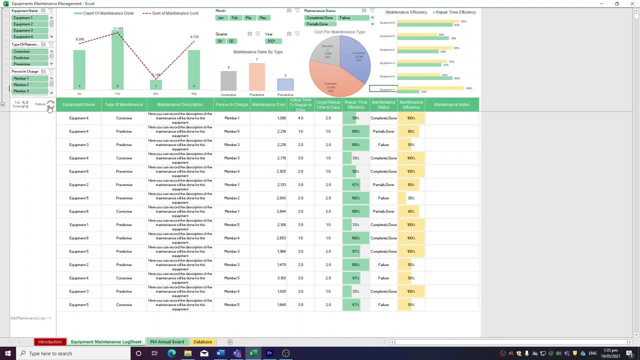 We have a refresh button to refresh the chart areas whenever you input any new data in the sheet. That's all for this template. If you want to automate your Excel processes and enhance your level of productivity, SimpleSheets, Advanced Templates and University is the best tool out there.